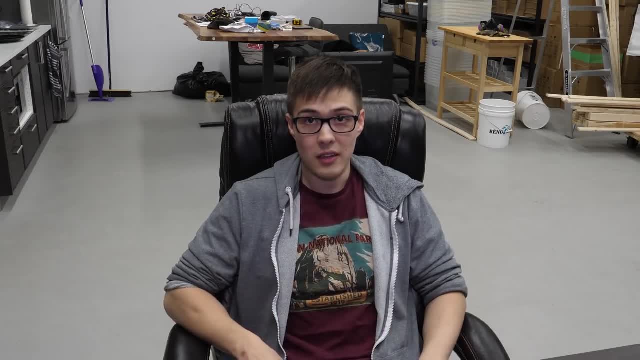 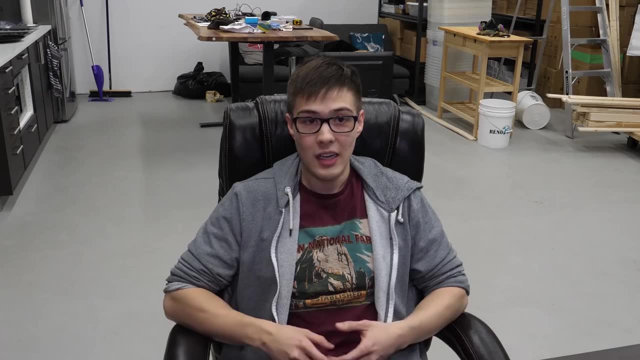 one yet. You have to just progress slowly and eventually you'll make it there. I get a lot of questions like this, where people want to know they're like I'll have $2,000. I can. just what should I buy? I don't even have an answer for that. You just buy what you need and do it. 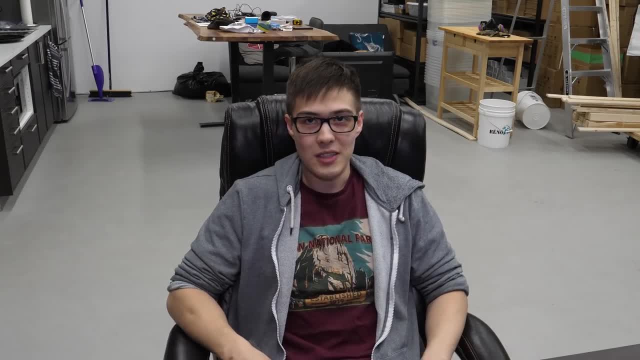 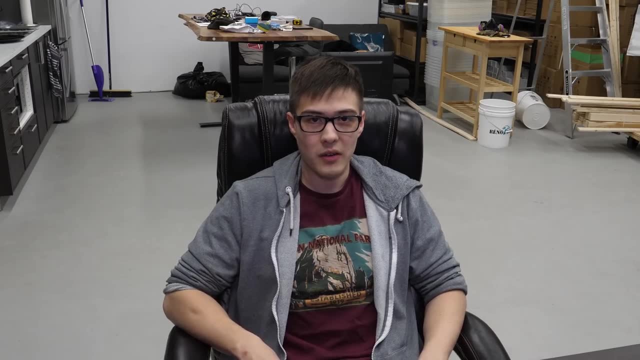 If your project's $2,000, then go ahead, But it's kind of like an expensive thing to start with. But with that being said, I there is one other thing that I wanted to talk about, and it's I'm- I've always, I'm answering this question to help people out. 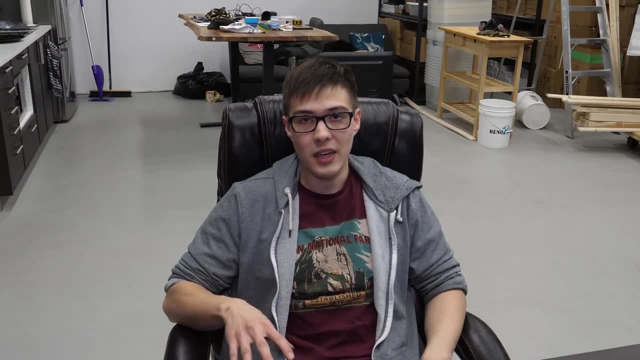 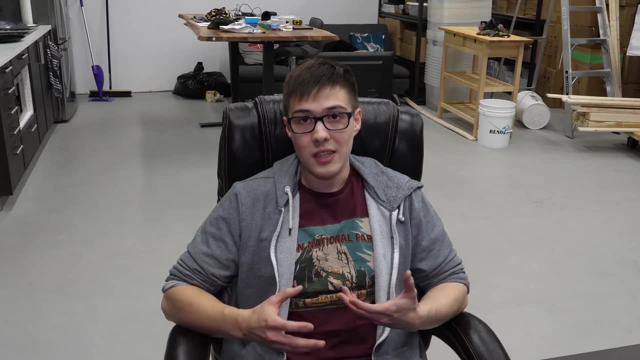 for them to get started. but I've always- I've always- kind of been a bit uncomfortable encouraging people to do chemistry on their own, because I don't necessarily make it that clear in my videos. but it's a very dangerous thing to do If you don't know what you're doing. 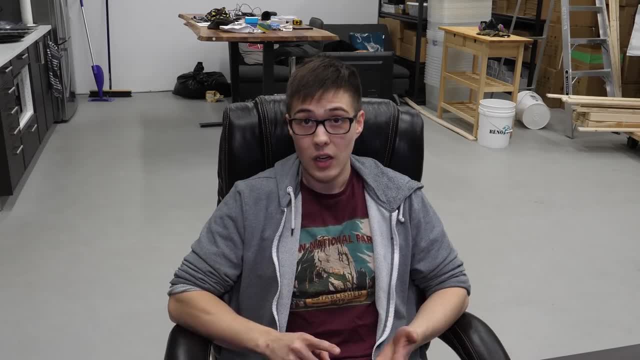 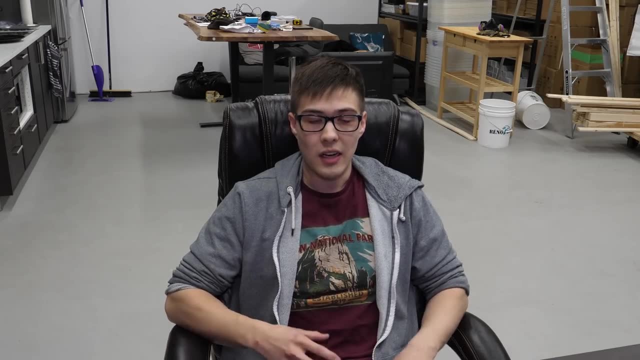 you can make a lot of mistakes where you can either hurt yourself or other people, And it's something that you really have to take into consideration And I don't in my videos- I don't want to be a drag and you know hammer and all these negative things and dangerous about. 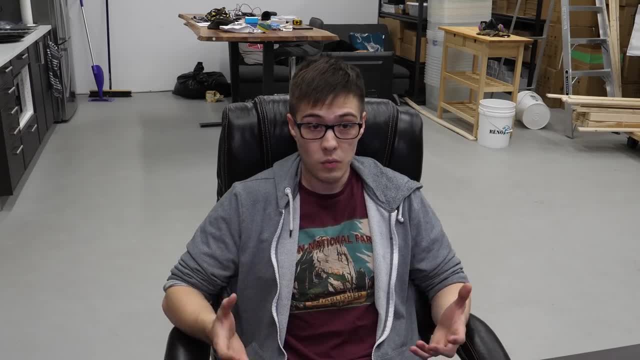 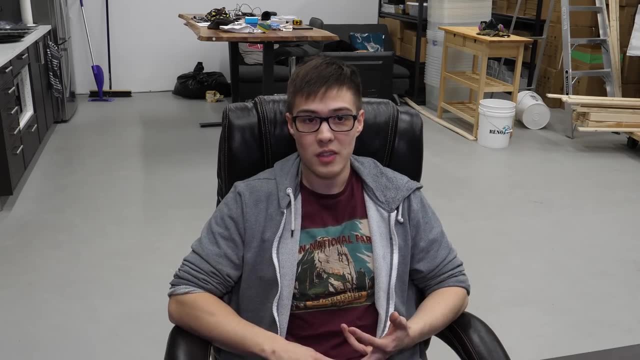 chemistry, but that is kind of the reality of it. Uh, when you decide to do a hobby like chemistry, it's dangerous. It involves toxic chemicals, corrosive chemicals, And you know if you have gases those are really dangerous chemicals. And you know if you have gases, those are really. 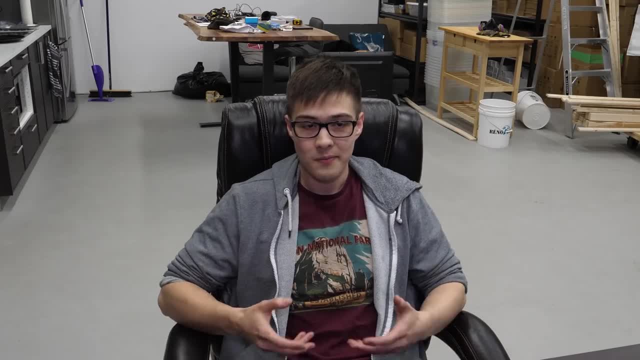 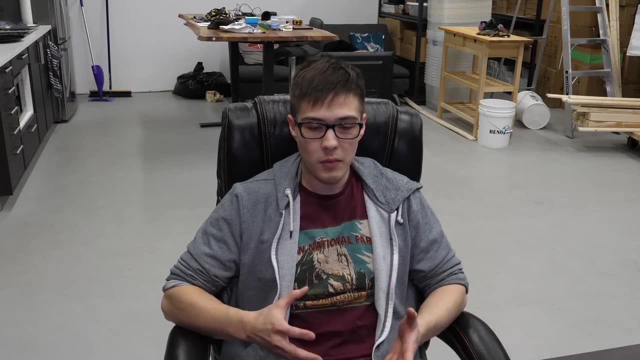 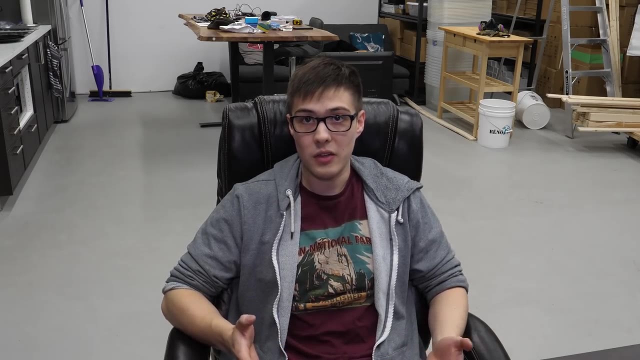 really bad, And you can also have fires, And these are all things to take into consideration. So it's I- really I'm at this weird place where I really do want to encourage people to experiment on their own. It's something that I did since I was probably like eight or 10, and it's what led 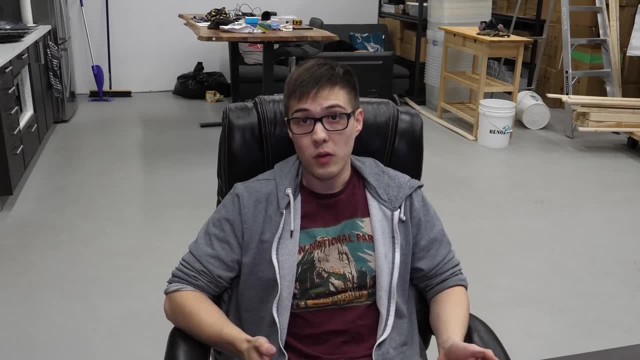 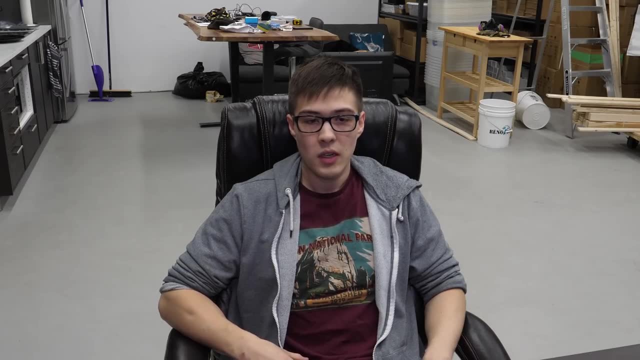 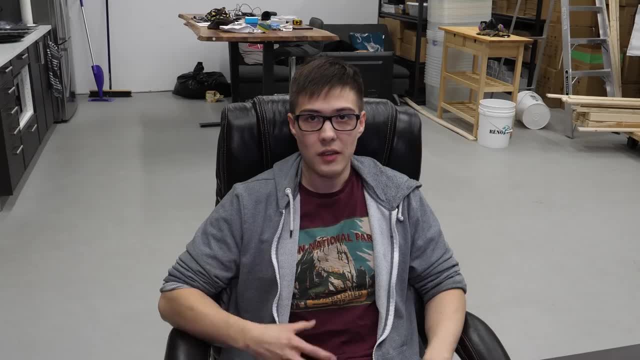